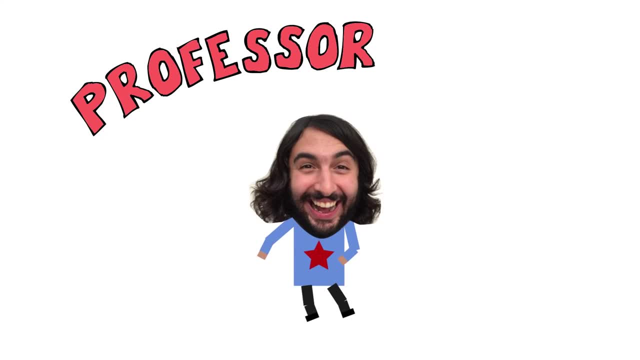 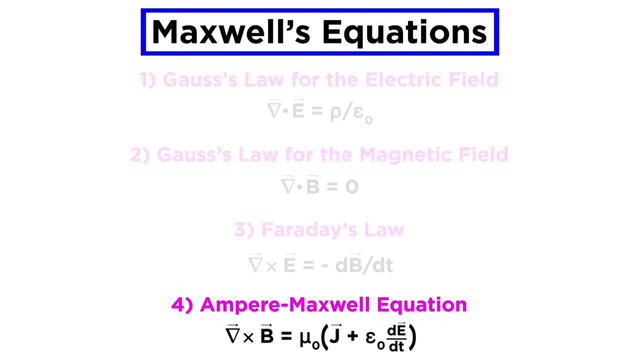 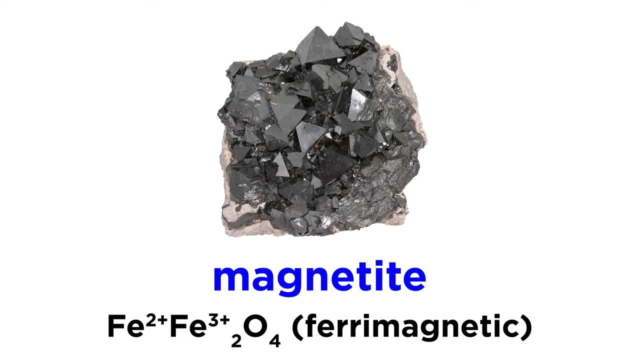 With three of Maxwell's equations covered. there is just one more to go. But before we dig into it, let's get through some background information. For the vast majority of human history, the only known sources of magnetic fields were certain iron ores and other materials that were. 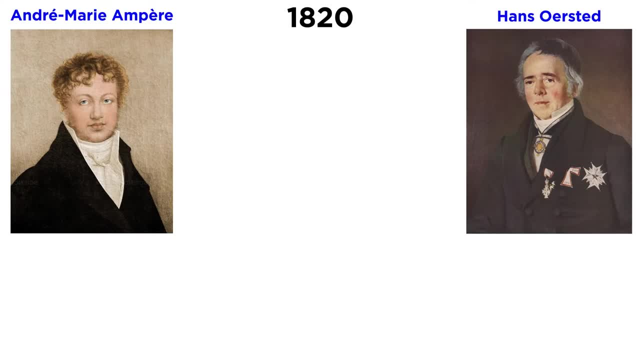 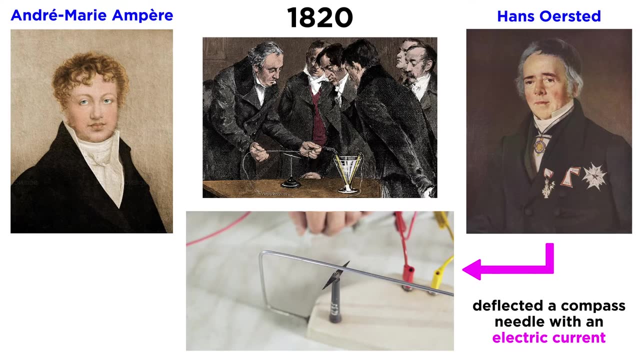 magnetized in one way or another. In 1820, French physicist André-Marie Ampère heard that in Denmark Hans Oersted had deflected a compass needle by passing an electric current nearby. Within a week, Ampère had begun quantifying the relationship between electric currents and the 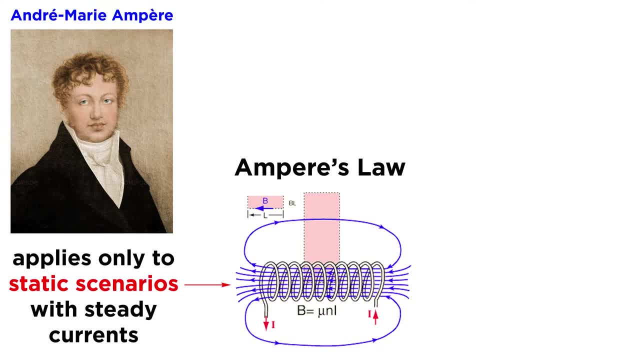 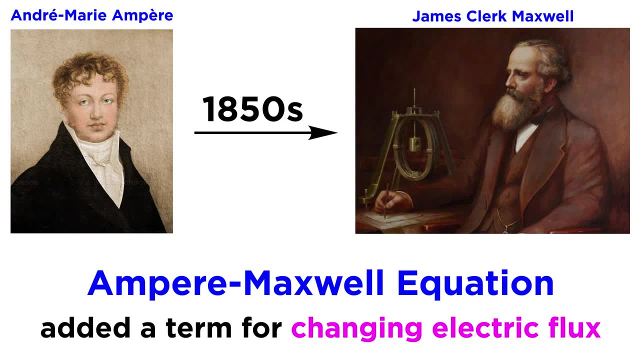 magnetic field. For many years Ampère's law was known to apply only to static scenarios with steady currents. Maxwell's addition of a new term for changing electric flux in the 1850s allowed Ampère's law to apply to time-dependent situations. 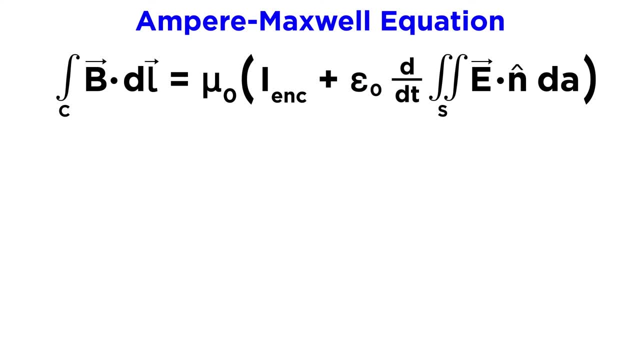 Here is the integral form of the Ampère-Maxwell equation. Let's unpack this a little bit before applying it. The left side represents the circulation of the magnetic field along a closed path C. The right side is divided into two parts: the electric current, I. 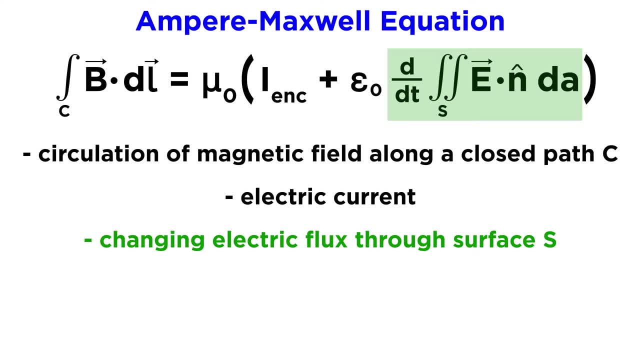 and the changing electric flux through a surface- S, which is this whole term over here, And we also have the permeability of free space, represented by mu naught. This difference comes from the other term we are familiar with, epsilon, which was the permittivity of free space. 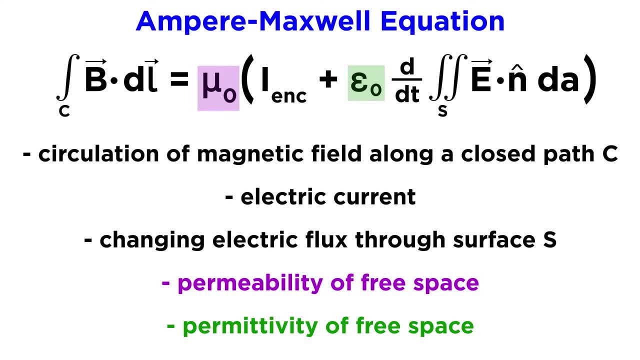 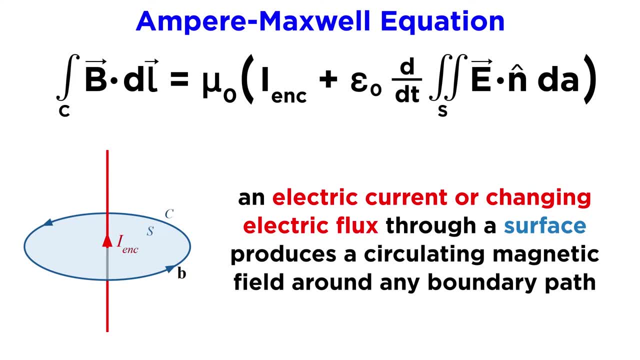 Permeability of free space deals specifically with magnetic fields. The main idea of this equation is that an electric current or a changing electric flux through a surface produces a circulating magnetic field around any path that bounds that surface. This idea is rather similar to the other three equations, The way the magnetic field term is surrounded by. an integral is the same as the other three equations. The way the magnetic field term is surrounded by an integral is the same as the other three equations. The way the magnetic field term is surrounded by an integral is the same as the other three equations. The way the magnetic field term is surrounded by an integral and a dot product. 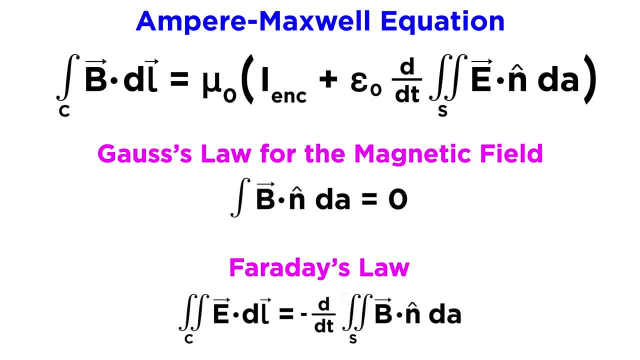 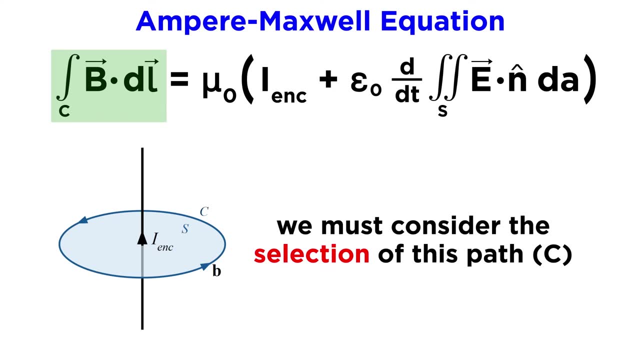 echoes the structure of Gauss's law. The law itself is almost a mirror of Faraday's law. Instead of a changing magnetic field leading to a circulating electric field, we see a changing electric field leading to a circulating magnetic field In many Ampere-Maxwell problems. the main consideration. 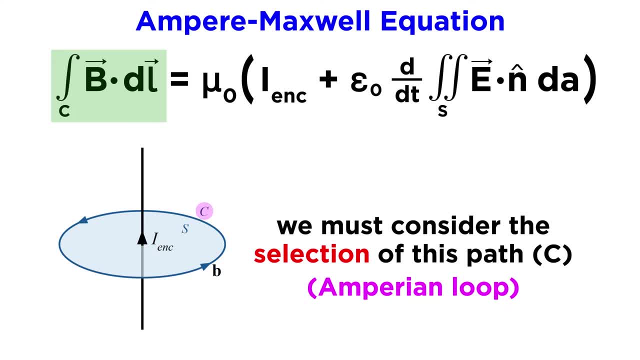 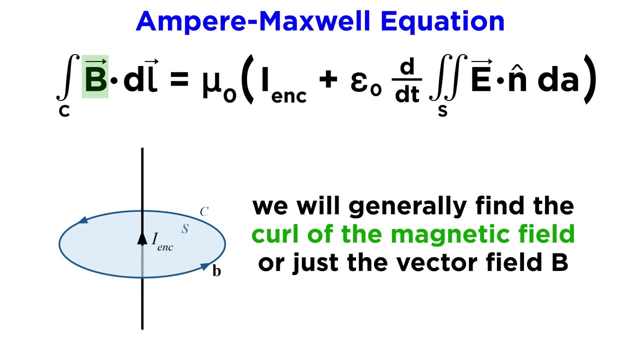 is the selection of this path, often called an Amperian loop, careful consideration that takes advantage of any symmetrical element. The solution to this problem is to use an amperian loop, or an amperian loop to determine the magnetic field, of the magnetic field or the magnetic. 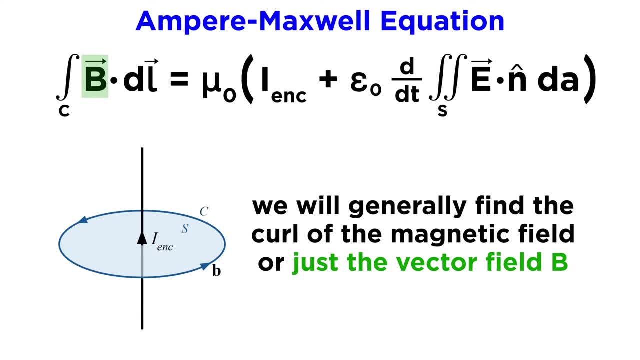 field directly from a current meaning just the vector field B. It is rare to see it used in the other direction to find the electric current from the circulating magnetic field, due to the dynamic nature of the two electrical terms. on the vector field B. 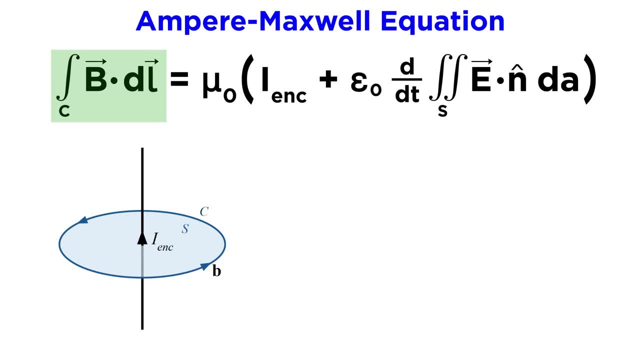 Like the electric field in Gauss's law, the magnetic field in Ampere-Maxwell is buried inside an integral and coupled to a vector via a dot product. This further implies that a high level of symmetry is required to determine the magnetic field from the electric current or a changing. 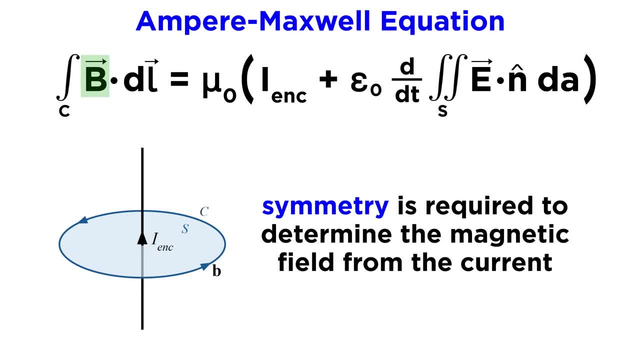 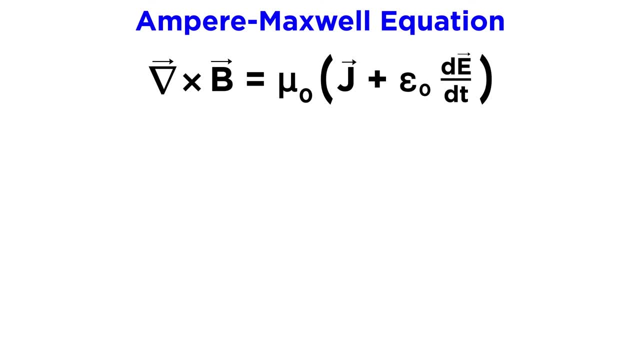 electric flux. The challenge arises in finding a way to move the magnetic field term out of the integral. The differential form of the Ampere-Maxwell term is the magnetic field term or the magnetic flux. The Ampere-Maxwell law is more often used in the opposite direction of the integral. 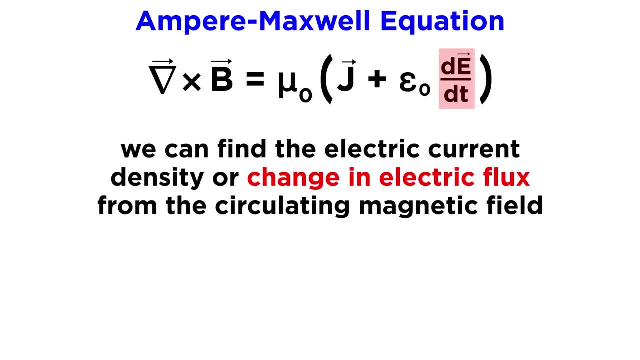 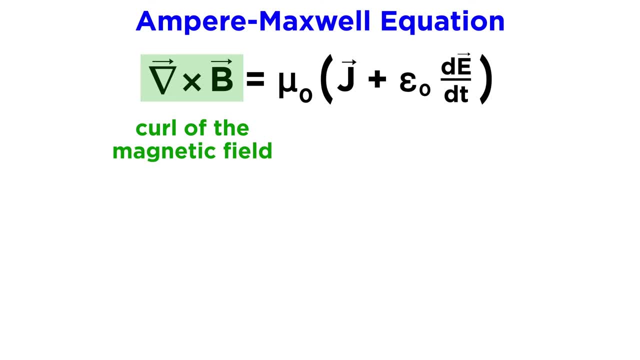 form to find the electric current density or change in electric flux from the circulating magnetic field. This form looks like this, with the cross product or curl of the magnetic field on the left and then this other term on the right: Mu-naught is back again, which. 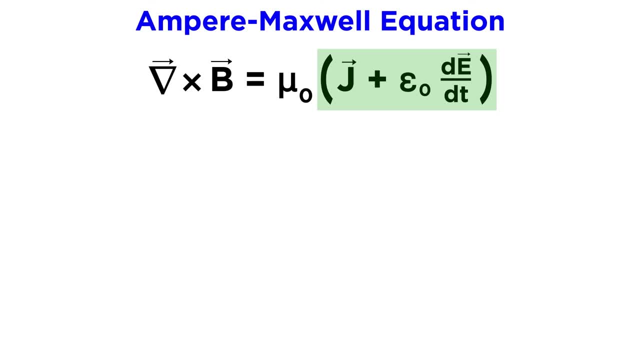 is the permeability of free space times. this sum J is the current density, and then we have epsilon-naught, the current density, which is the current density of free space times. this sum J is the current density, and then we have epsilon-naught. 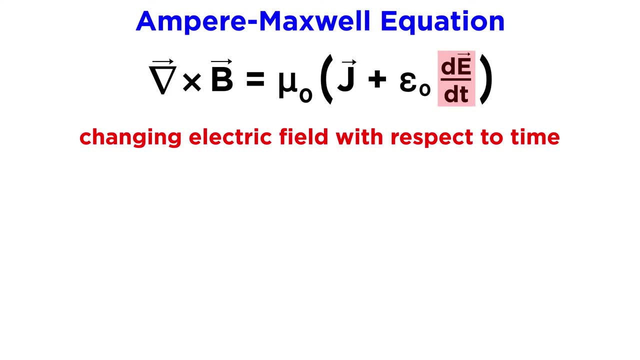 the permittivity of free space times, the changing electric field with respect to time in the region in question. These generally can't be determined from the curl. at the same time, they have wildly different influences on the equation and mathematically separating.